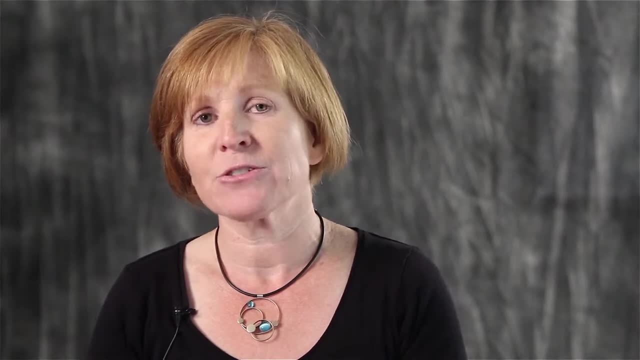 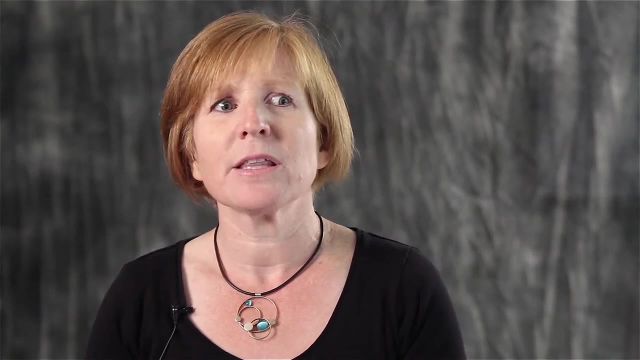 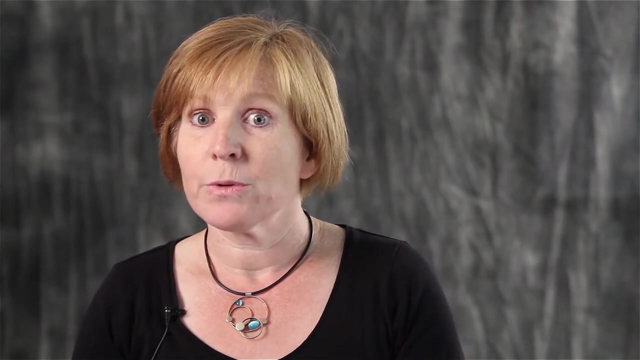 teach it so they can work with the students in the elementary classrooms. Teaching mathematics has changed so much in the past 20 years and teachers are really struggling to keep up with what these changes need to look like in their classrooms. My research has shown that elementary pre-service teachers really struggle with fractions and decimals and measurement. 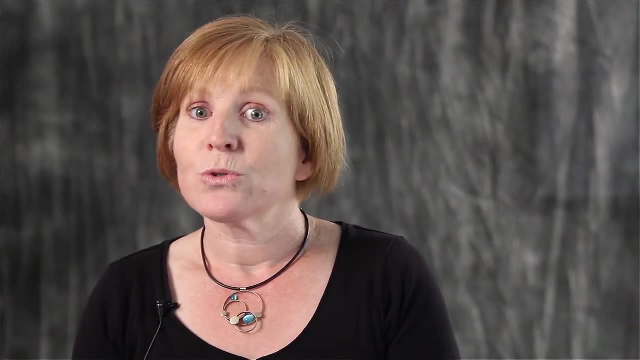 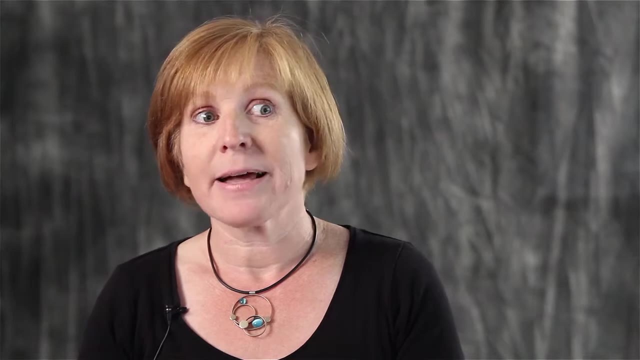 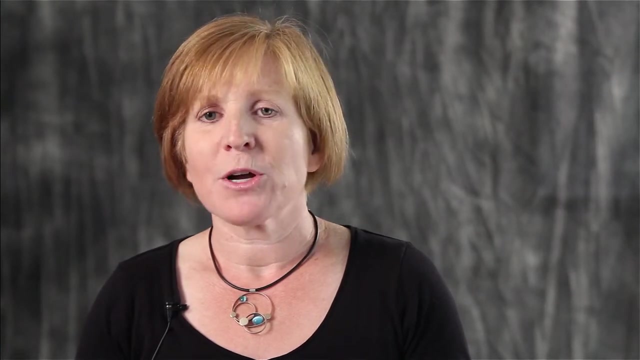 So what I've been working on is trying to develop learning tools and various teaching strategies that would support these teachers as they move forward in their understanding of mathematics. Research is so strongly connected to my teaching practice. Each year I make major modifications in the courses. I create new learning tools. 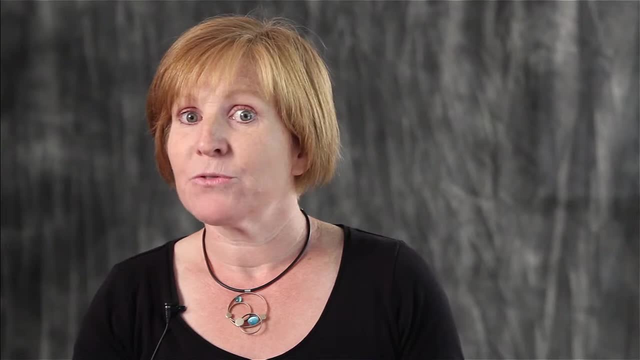 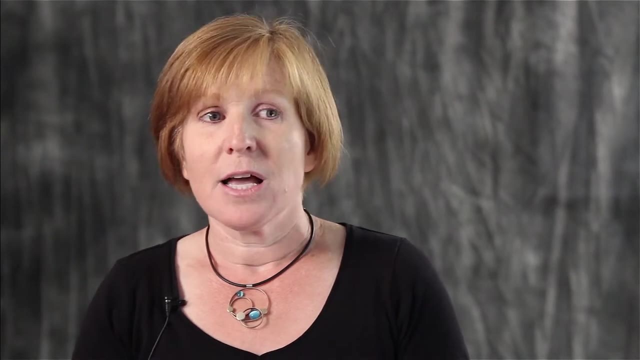 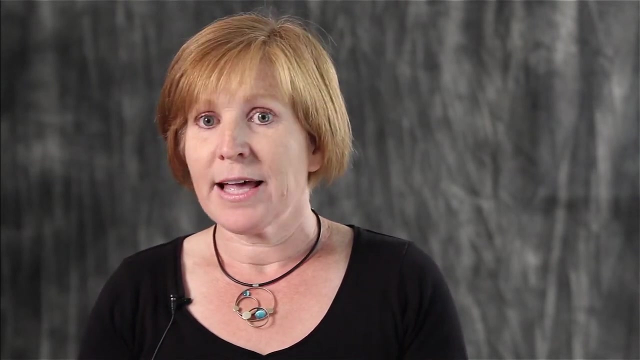 I create new resources based on the information I collected the year before. So, for example, I was working on developing a diagnostic assessment for pre-service teachers to figure out: okay, this is what they know in content, this is what they don't know. So, discovering that, 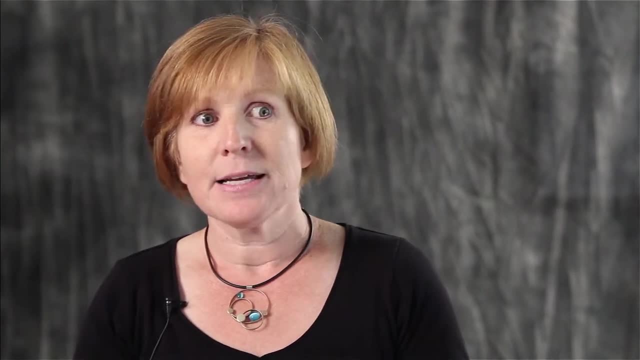 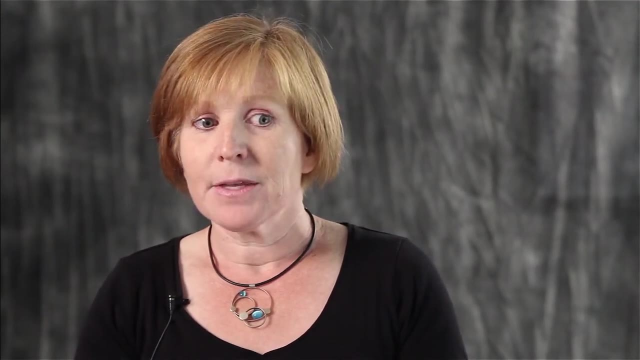 I made major changes in my course. I developed some video clips, created some websites that focused on those concepts And then to watch over a very short period of time and then looking at pre-service teachers using those instruments and saying, wow, that was effective. 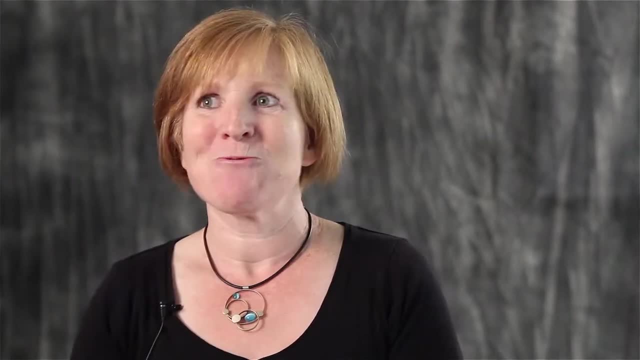 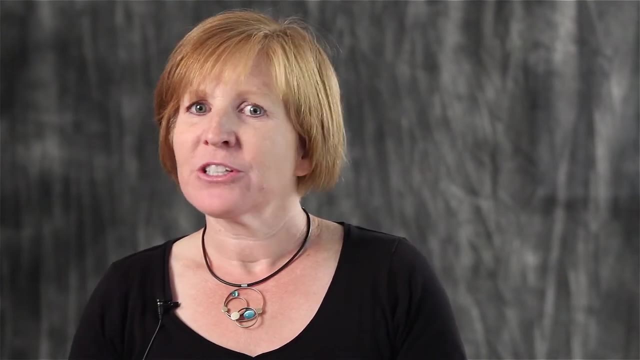 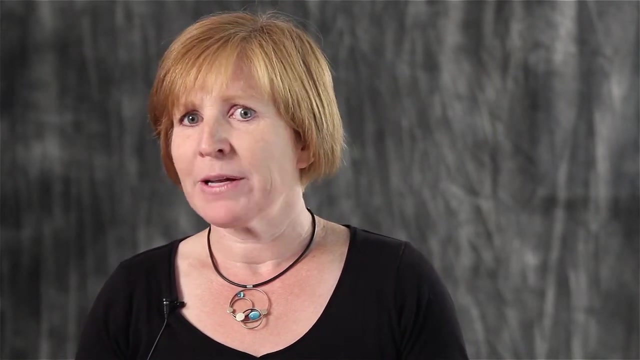 That worked for me, So for me that was huge. If we can work with teachers, pre-service teachers and practicing teachers and start to change their conceptions of mathematics and their confidence in teaching and learning mathematics, then they will have a broader 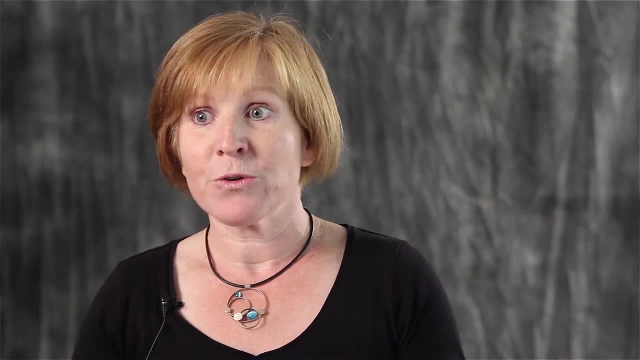 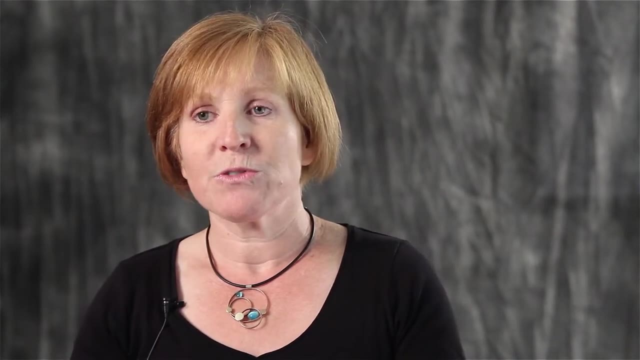 impact on the next generation of children coming through our elementary school system, And that has grand implications for the future of our school system and the future of our school system, Our entire society, which is already a strongly math, computer science-based society. So 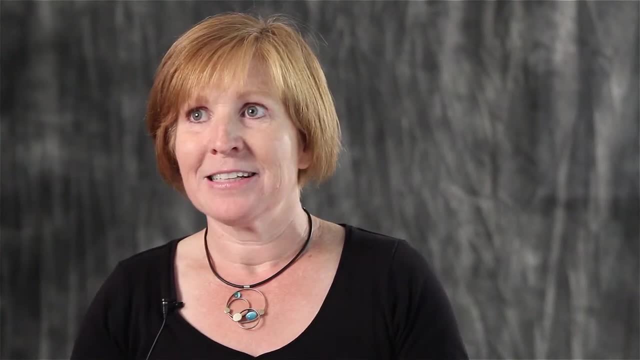 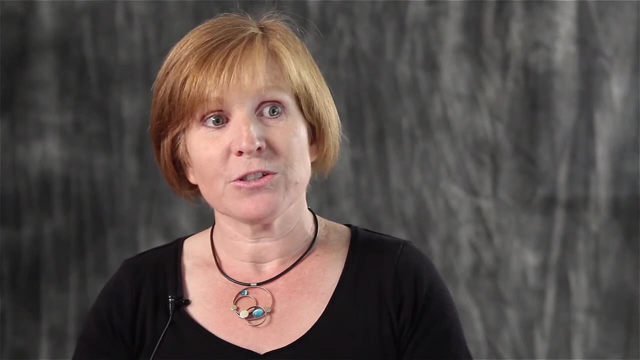 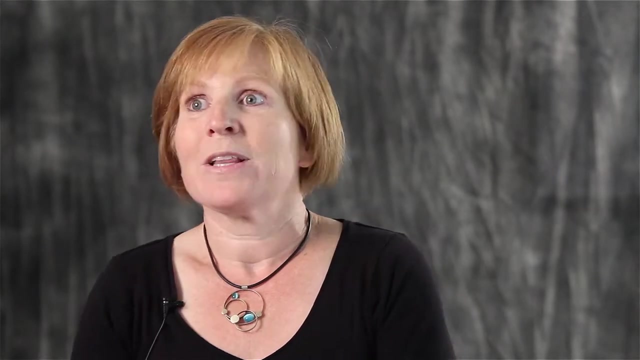 if we can graduate students that are confident in their mathematics skill sets and confident as learners of math and problem solving when they move into the greater society, we could have a generation of kids who are broader thinkers and willing and able to make huge changes in the future. 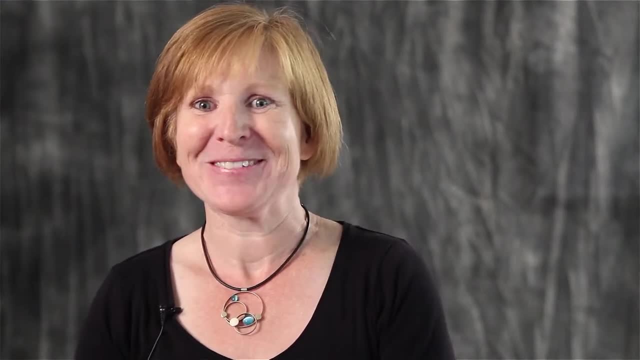 That's a big grand idea. I'm not sure if that'll actually happen, but ideally that's what I'd be looking for. That would be wonderful.